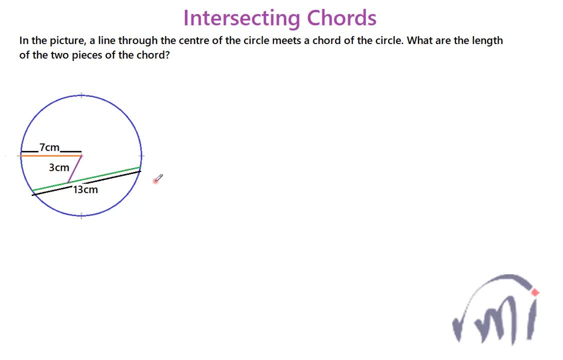 of two pieces in which this chord is getting divided by this line. So to solve this problem I'm going to use the intersecting chords theorem, where these lengths are in particular ratio. So first let's learn what that theorem is and then we will use that theorem to solve this problem. So 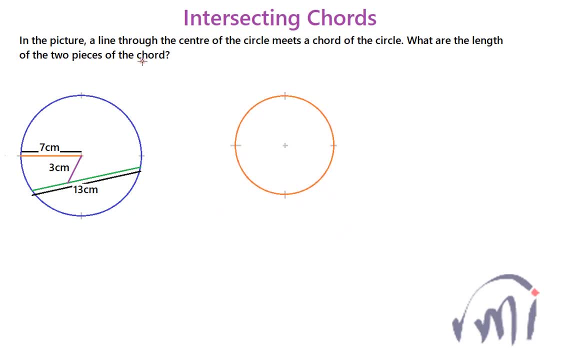 to know what intersecting chords theorem is. I have again made a picture of a line through the center of a circle which is seven centimeters, and a line made a circle, and in this circle I'm going to draw two chords. So let this be one chord and let this 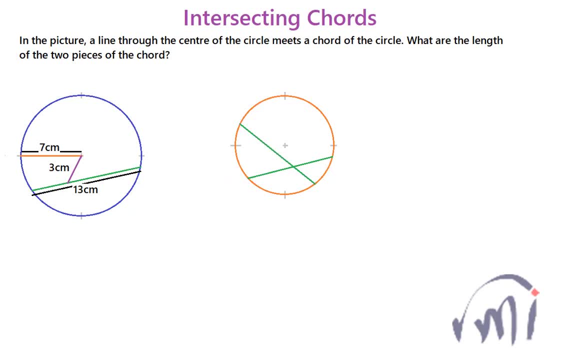 be another chord, and these are two chords which intersect each other at this point. So let this O be the center of the circle and let me call this point of intersection as point B. Let this be the chord AB and let this be the chord CD, right? So what can you see Here? this angle, angle. 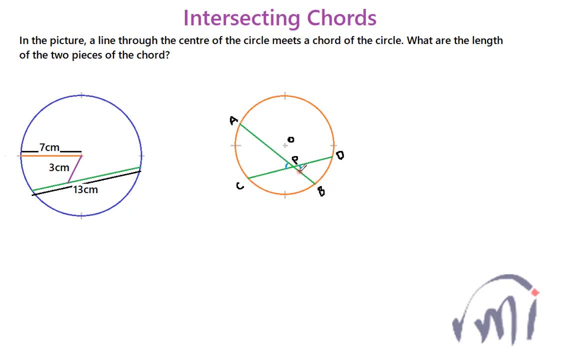 APC is equal to this angle, angle BPD. and now what I'm going to do is I'm going to draw a line from this point till this point and I'm going to draw another line from this point till this point. So now we have got two triangles: We have triangle APC and we also have triangle BPD. These two 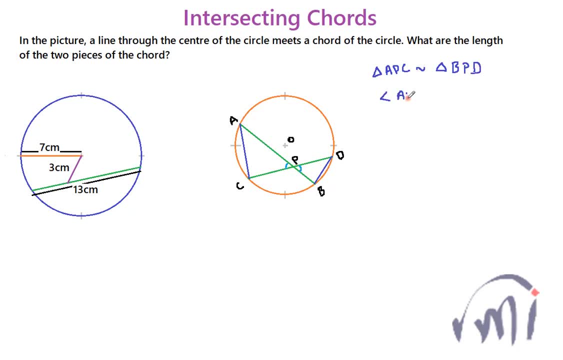 triangles are similar because angle APC is equal to this angle and angle BPD is equal to this angle. So angle APC is equal to angle BPD. These two are vertically opposite angles and at the same time, this angle is equal to this angle because both these angles are subtended by the same arc, CB. 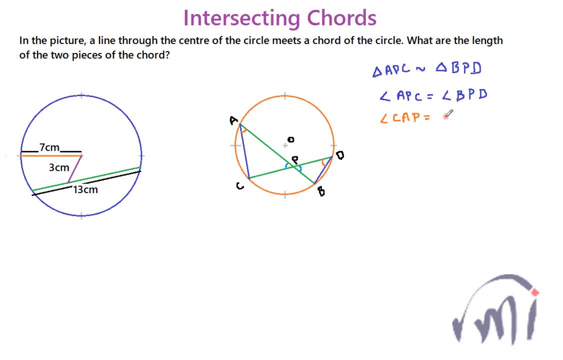 So we have angle CAP is equal to angle PDB. and we also have this angle is equal to this angle, because both these angles are subtended by arc AD, So the measure of those two angles will also be same. That means angle ACP is equal to angle. 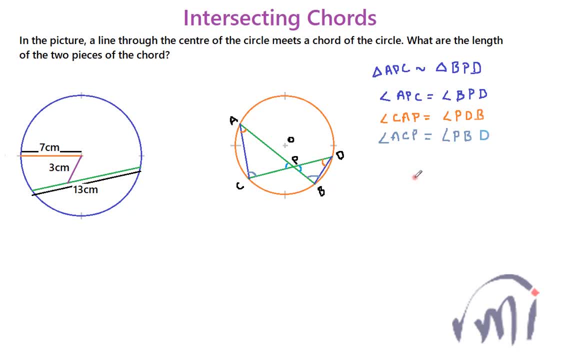 PPT. So since these two triangles are similar, that means PC by PB will be equal to AP by PT, corresponding sides of similar triangles. Since these two triangles are similar, so the ratio of CP is to PB will be same as the ratio of AP is to PD. 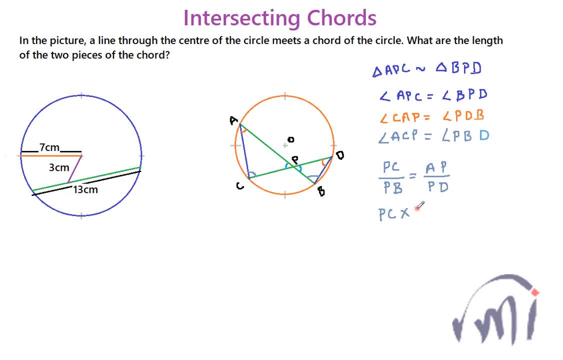 Here is what I have written here. That means PC multiplied by PD will be equal to AP multiplied by PB. That means the point where these chords are intersecting. if that is P, then AP multiplied by PB is equal to CP multiplied by PD. And this is the relationship of intersecting chords. 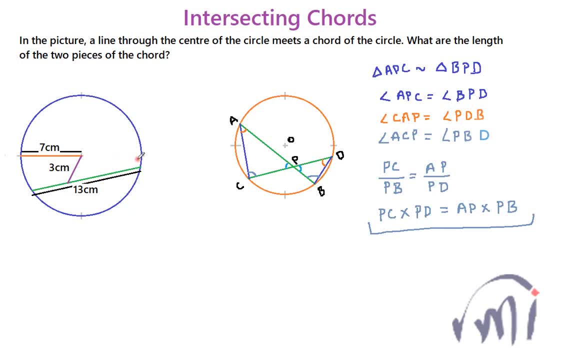 So this is what we are going to use over here and solve this problem. So let me erase all this. So let this be the center of the circle and let this be the chord AB and this point where this line from the center is meeting this chord, Let it be point P. Point P is actually. 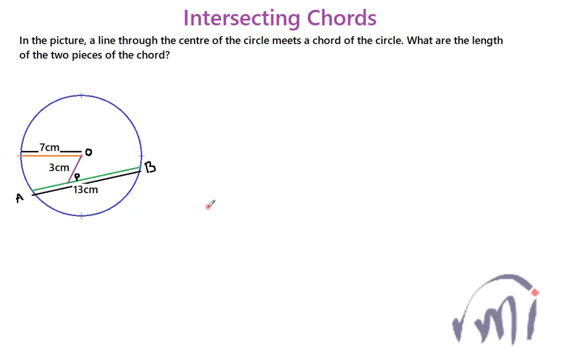 this point. So what we have to do, How are we going to use this theorem? So what I am going to do is I am going to extend this line, This line OP, I am going to extend in this direction and I am also going to extend this line in this direction. Now, let me call this diameter of the circle. 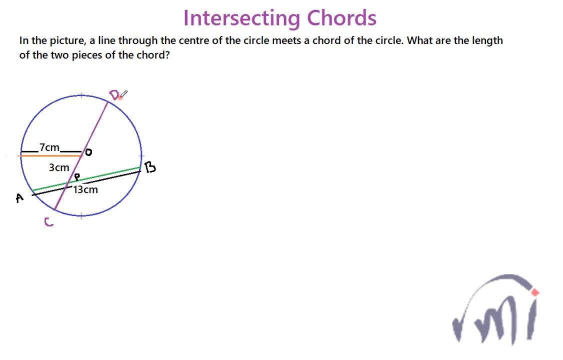 Since this line is passing through center O, this will be the diameter of the circle- Let me call this as CD- and diameter of the circle is actually the longest chord of any circle. So now we have two chords, AB and CD, and these two chords are intersecting each. 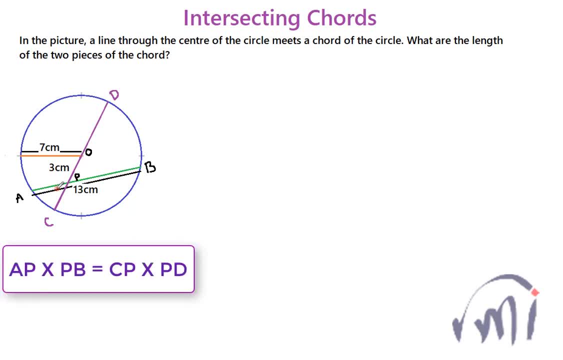 other at point P, And now we have to find the length of AP and PB. So if I assume AP is equal to X, PB will be equal to 13 minus X, And since we know the radius of the circle is 7 centimeters. 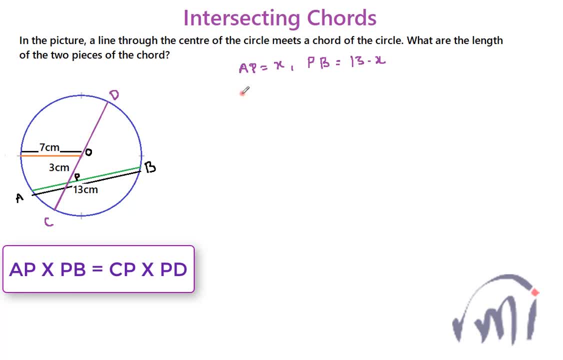 so OD will be 7 centimeters and PD will be equal to OP plus OD. OP is 3 centimeters and OD is the radius of the circle, which is 7 centimeters. So this will be equal to 10 centimeters and PC will be equal to OC minus OM. 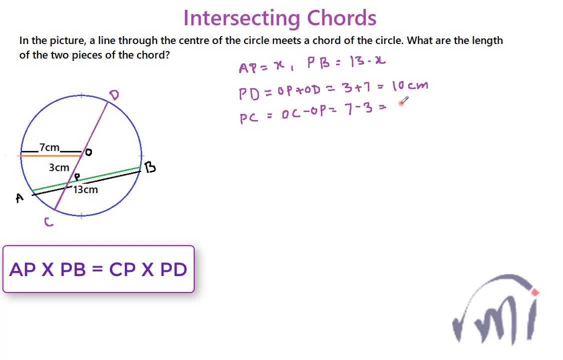 So we have 4 P, which will be equal to 7 minus 3, that is, 4 centimeters. And now we can use the property of intersecting chords. So CP multiplied by PD will be equal to AP multiplied by PB. So CP or PC is 4 centimeters, PD is 10 centimeters. this will be equal to AP, which.